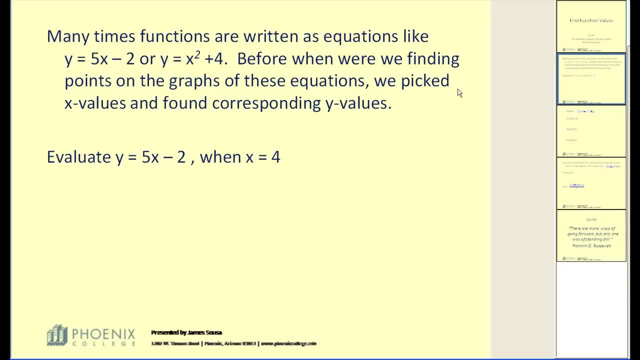 on the graphs of these equations. we picked various x values and found corresponding y values. Here's a simple example: Evaluate: y equals 5x minus 2 when x equals 4.. We know the process is essentially to substitute 4 in 4x and evaluate, So we have y is equal to 18.. 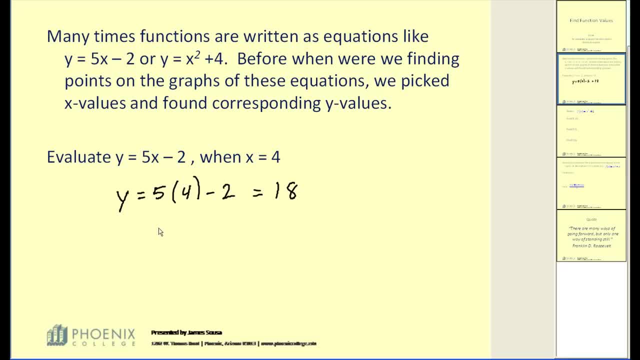 There are several ways to express this relationship. One way would be to write it as an ordered pair: When x is 4, y is 18.. With the new language of inputs and outputs that come with functions, we could say that when the input 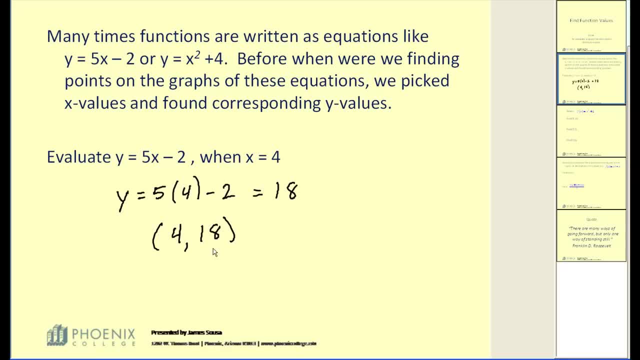 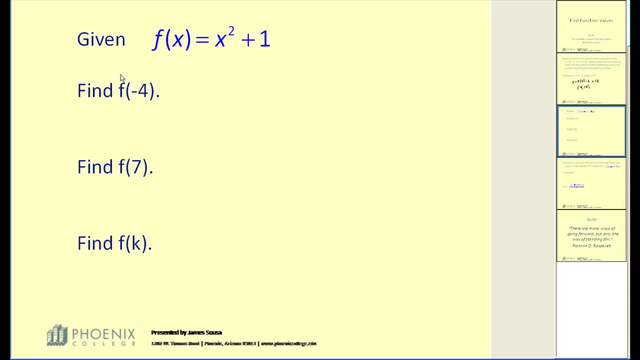 is equal to 4, the output is equal to 18.. We substituted 4 in for x. x is our input and y was equal to 18.. y was our output. Let's combine this thought with functions. Let's say that we're given f of x is equal to x squared plus 1. 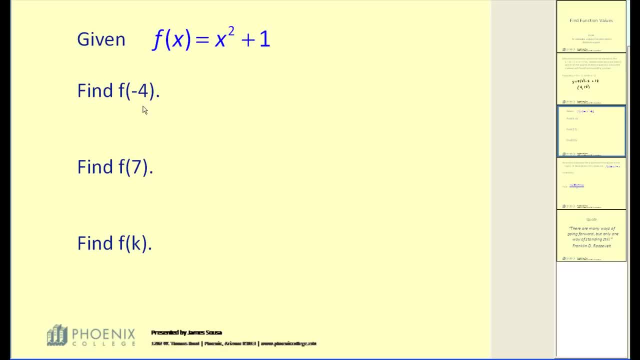 and we're asked to evaluate f of negative 4.. Negative 4 is our input. Let's take a look at this notation, though. Notice how this x has been replaced with negative 4, and that is essentially how you evaluate f of negative 4.. You replace or substitute x with negative 4.. 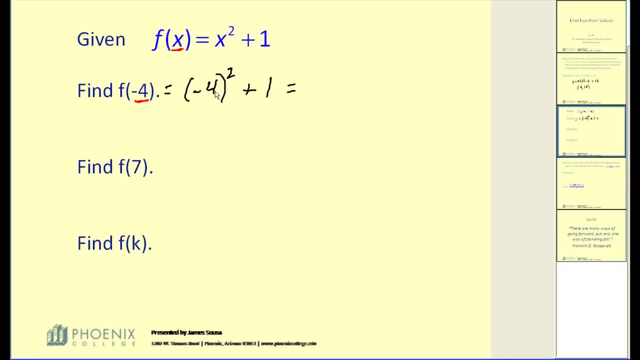 Negative 4 squared plus 1 gives us 16 plus 1 or 17.. So f of negative 4 is equal to 17.. Negative 4 would be considered our input, 17 would be considered our output. I'd also like to make the connection that this represents one point on the graph. 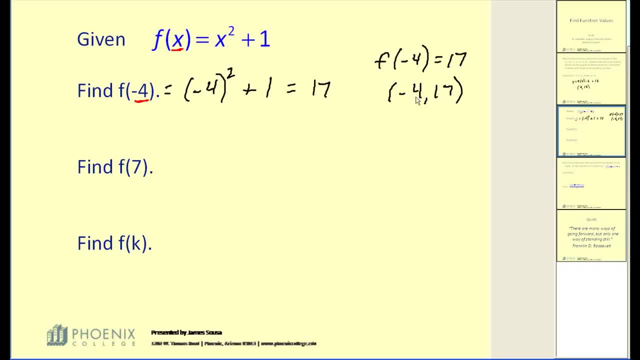 when x is negative, 4, y is equal to 17.. Most often, x is regarded as the input, y is the output. Okay, let's go on with another example: f of 7.. So this becomes 7 squared plus 1.. 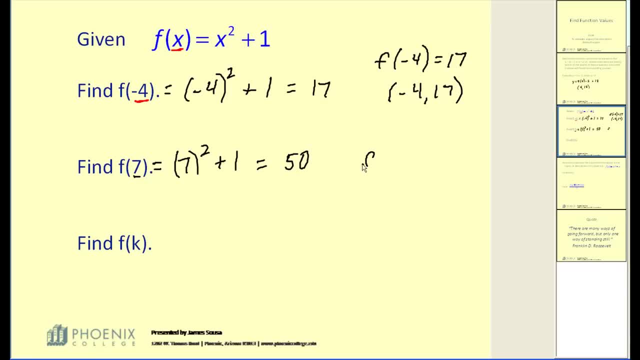 49 plus 1 is 50. So just to clean it up, f of 7 is equal to 50.. One more example: f of k. Now this may look a little confusing, but essentially we're going to be doing the same thing. 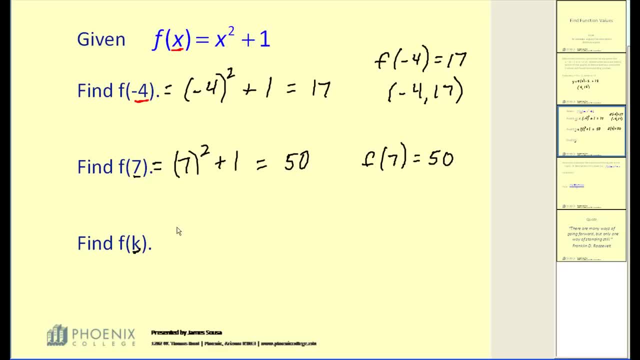 Now we're going to replace x with k- Same function. So f of k is equal to: instead of x squared, we have k squared plus 1.. Now we can't do anything else, because these are not like terms. Nothing's going to work. 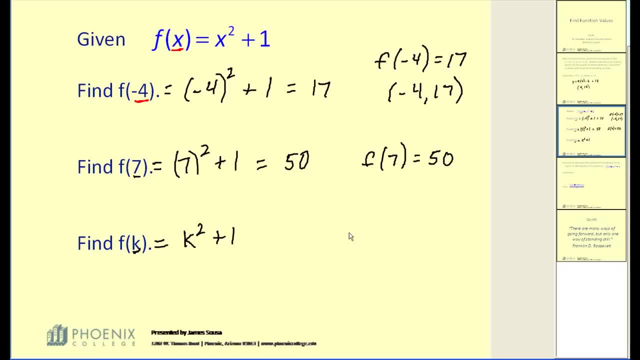 So f of k is equal to: instead of x squared, we have k squared plus 1.. Now we can't do anything else, because these are not like terms. Nothing's going to work. Something simplifies, so that would be our final. 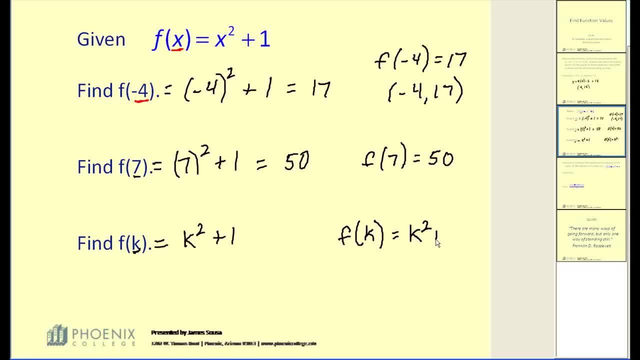 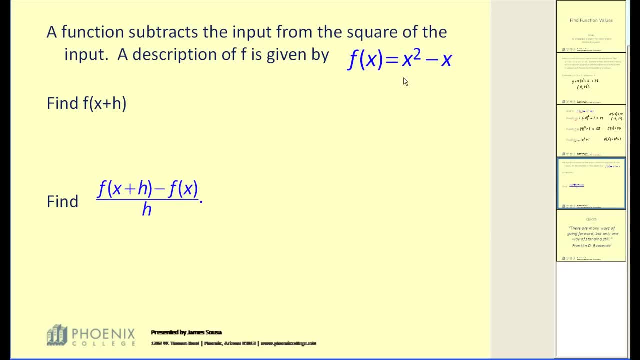 final form: f of k is equal to k squared plus 1.. Let's take a look at a couple more involved examples of evaluating functions. A function subtracts the input from the square of the input. A description of f is given by: f of x is equal to x squared. 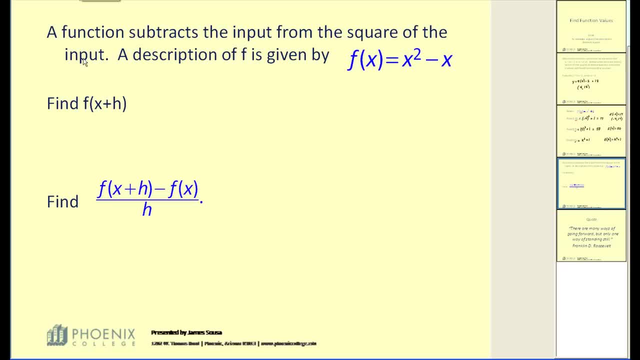 minus x. Our goal is to find f of x plus h. our goal is to find f of x plus h. our goal is to find f of x plus h, or in other words, our input is X plus H. the question is, what would the output be? 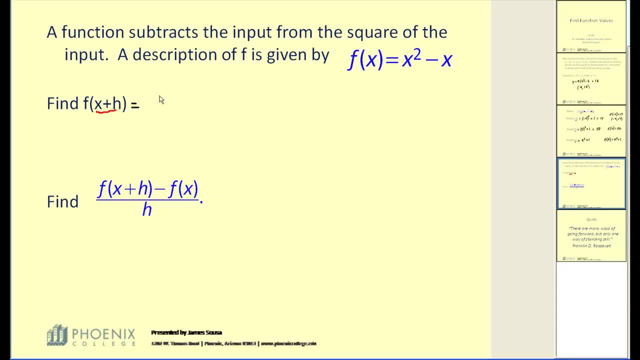 well, let's replace X with X plus H. so we're going to square it and then we're going to subtract it. okay, remember, there's no shortcuts to squaring X plus H. we have to write this out twice and foil it. that would give us X squared plus. 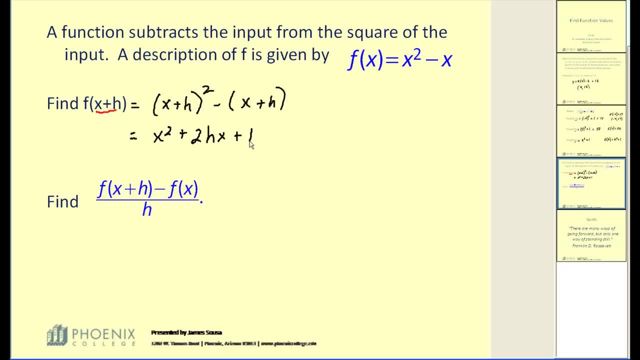 2, H, X plus H squared. you can check me on that if you'd like, by writing it out and multiplying it. next, we want to eliminate the parentheses. here we're going to subtract this quantity. some of you may have been taught to put of a, put a 1. 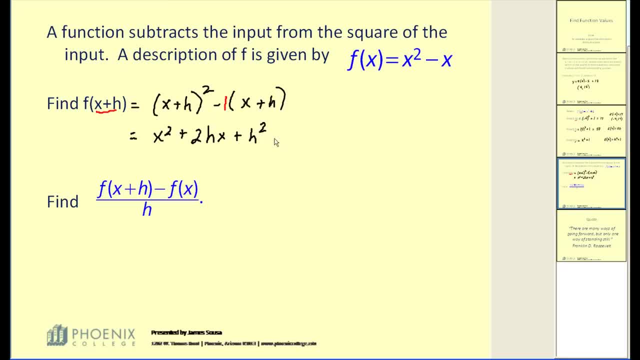 there and distribute a negative 1, whichever method you're used to doing. okay, go ahead and make sure that you get minus X, minus H, and in fact there are no like terms here. so we are done. f of X plus H is equal to the sum and difference. 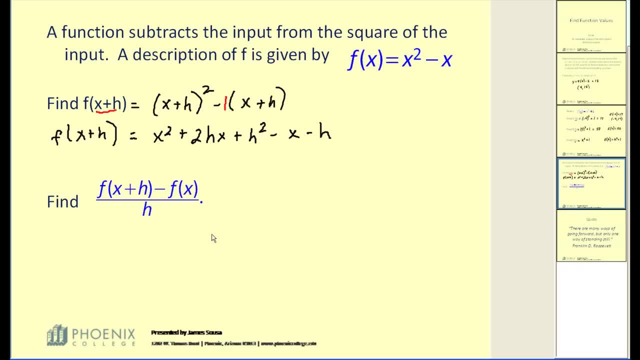 of all these terms. the last example I would like to take a look at. we want to find f of X plus H, minus f of X all over H or divided by H. okay, let's take this one step at a time. now this previous problems does give us f of X plus H. it gives us this: 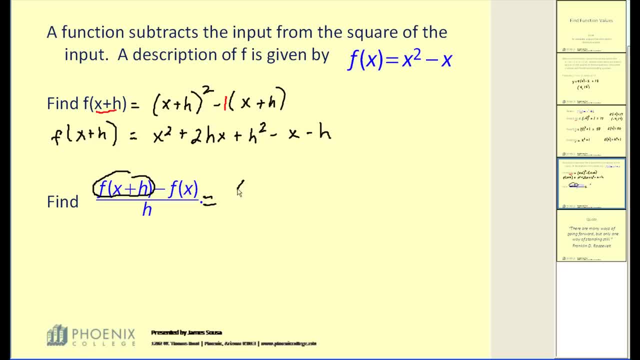 piece of this fraction. so let's rewrite that we have X squared plus 2 H, X squaredch kamiya minus H, minus slapi of X. we have to track the quantity x squared minus X. so if we subtract both of those terms we would get a minus Awakens. 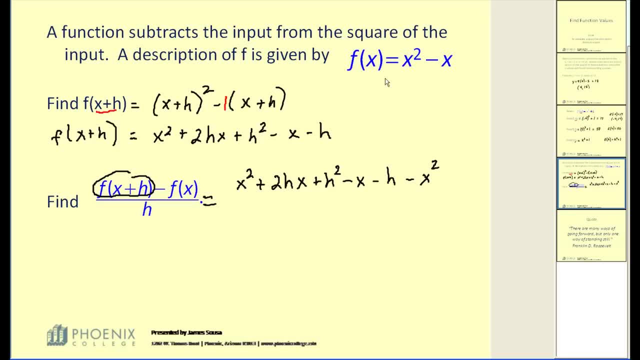 terms, we would get a minus minus x squared, And then, if we subtract a minus x, which that would be plus x, All of this would be over h. Notice we're not substituting h in, because they didn't give us f of h. 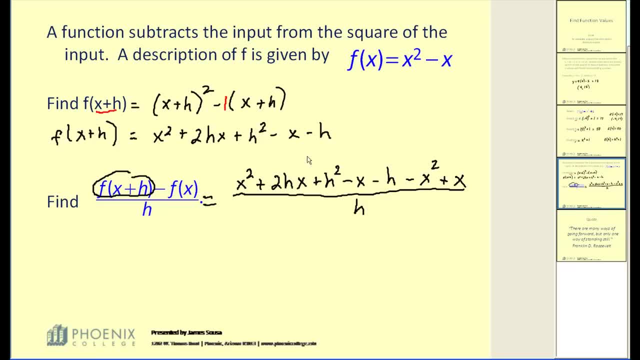 they just gave us the variable h. Let's see if we can simplify this. First off, let's look at the numerator and we'll notice there are some terms that are opposites. We have an x squared here minus x squared there. 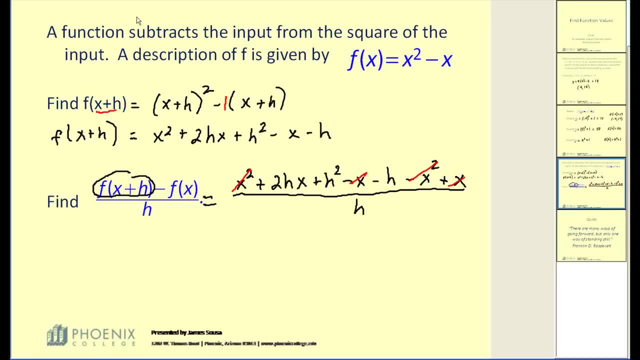 We have minus x plus x. Let's rewrite what we have so far. We have two hx plus h squared minus h. Now, dividing all of that by h: notice, they all have an h in common. so what I'm going to do is divide them. 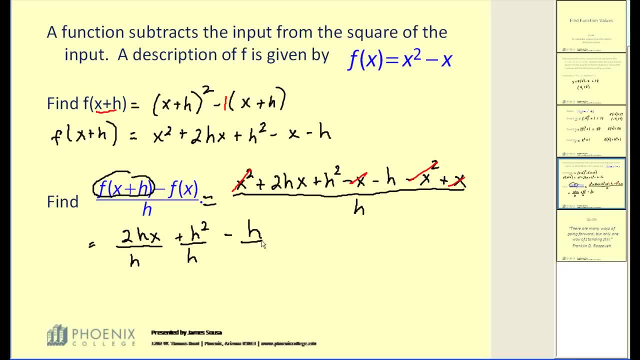 all by h. I'm going to simplify h individually. Remember you're allowed to do that as long as you're dividing by a monomial one term. And the reason I did that: it's very easy to simplify these. now. Notice how the common factor of h, here and here, 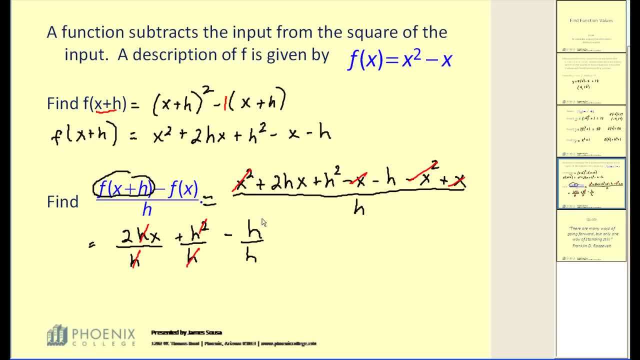 one common factor of h here. that would turn into h to the first power, and h over h would simplify it as well. So what's left? We have two x plus h, and then this is minus one, So this entire fraction. that involves the function notation. 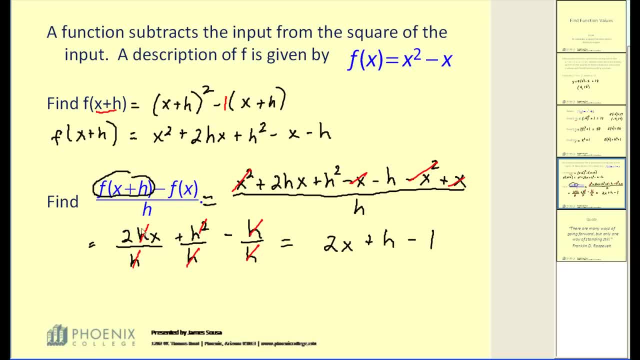 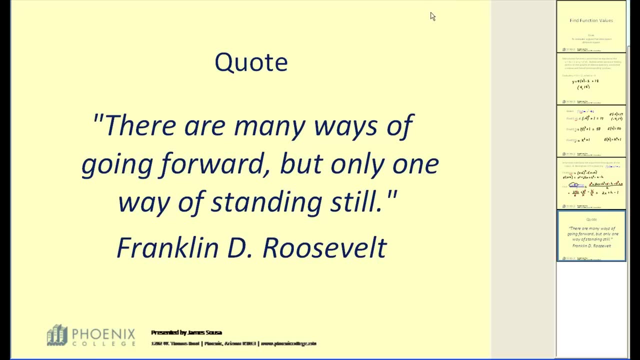 is equal to two x plus h minus one. This is actually called the difference quotient. that will show up later on in the semester. I hope that helps explain how to evaluate functions. Thank you, Thank you, Thank you.